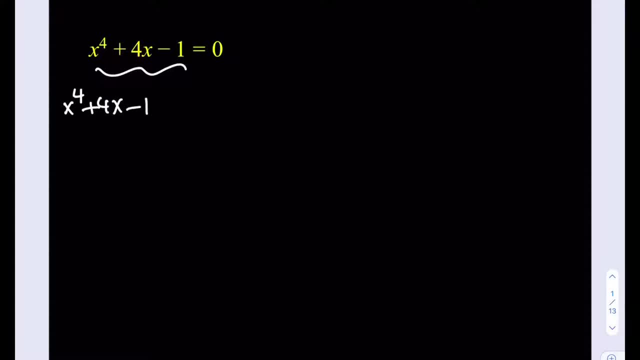 and I'm going to write it as a product of two polynomials, One of which is x squared plus a, x plus b. The other one is going to be x squared plus c, x plus d. Then what I'm going to do is I'm 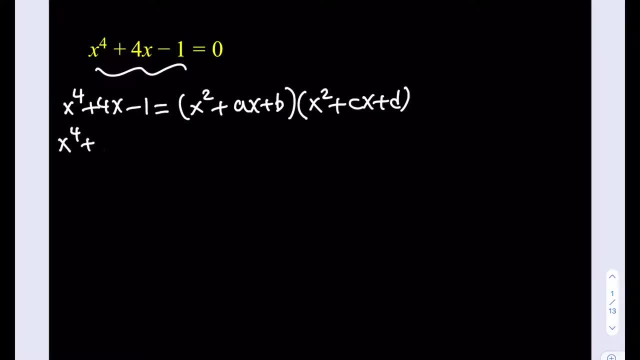 just going to go ahead and distribute on the right hand side and then set the coefficients equal to each other, so on and so forth. Let's go ahead and do that. We're going to get some interesting results from here. Okay, so if you distribute the x to the fourth term we're going to get, so they're going to match up. 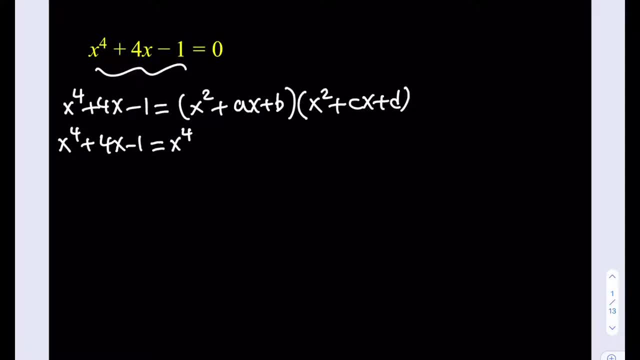 that's good To make it a little easier. let's go ahead and go by x powers. We get an x cubed. that's going to be like a x cubed plus c x cubed, so it's going to be a plus c x cubed, and then the 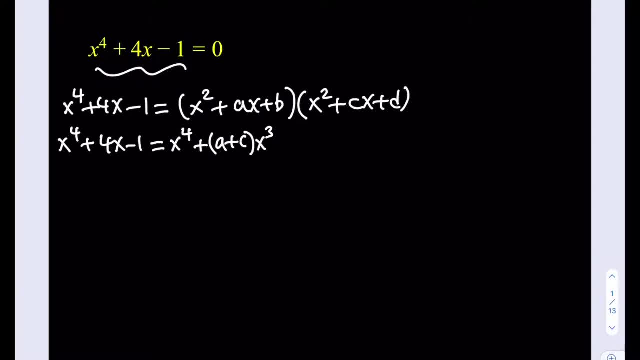 x squared. term is going to be: we'll get b x squared and d x squared and a c x squared. So if you put that together, it's going to look like a c plus b plus d times x squared, and then we're going to get 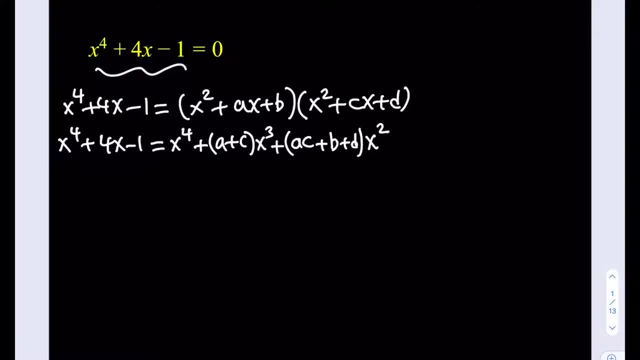 an x term, which is going to be like a- x times d and c x times b. So it's going to be a d plus b c times x, and then, finally, our constant is going to be b- d. Okay, so these two polynomials are going. 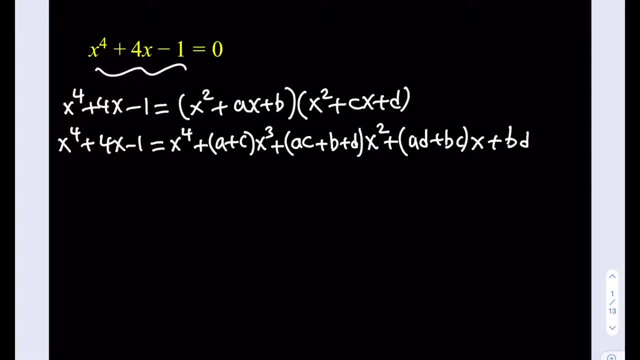 to equal each other for every x, Meaning that we can kind of determine the coefficients here. So from here, a plus c. there's no x cubed term, so a plus c is going to be zero. There's no x squared, so this is also going to be. 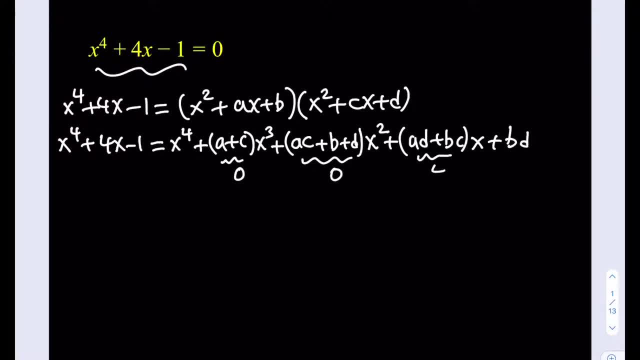 zero. The coefficient of x is four, so this is going to equal four and our constant is going to be negative one. And we are looking for integer a, b, c, d here. so hopefully we're going to find some- or maybe they're not integers, we don't know yet right, But the product b d equals negative one. 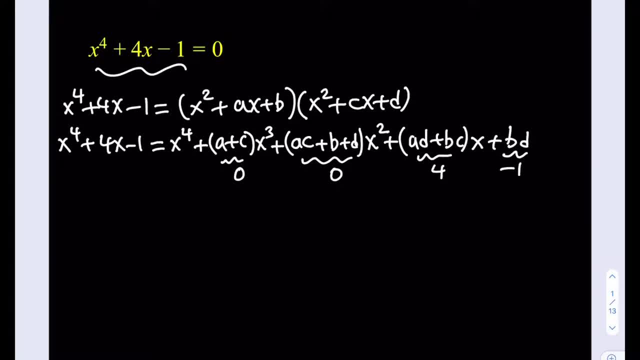 tells me that it can be plus minus one, but we do not know if they are integers, So we can't really assume that, Anyways. so let's go ahead and write this down: We have a plus z equal to zero. a, c plus b plus d. 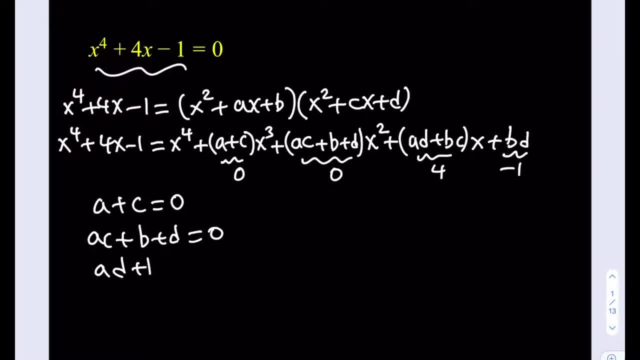 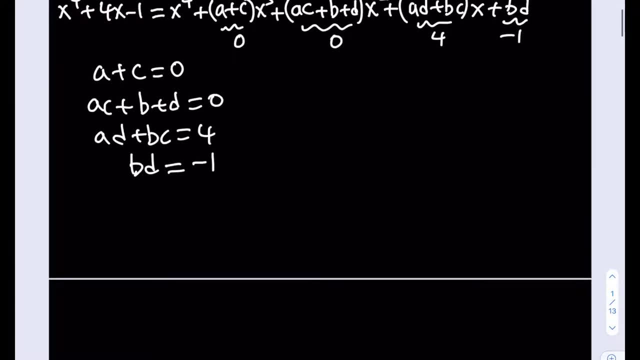 equal to zero. a d plus b c equals four and b d equals negative one. Okay, all right, so that's kind of like a system of equations and there are four variables. so we should be able to solve this right. I mean, it should not be too hard. Okay, so from here you can just go ahead and actually eliminate. 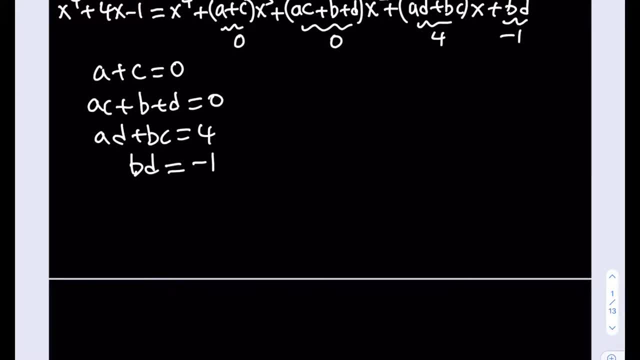 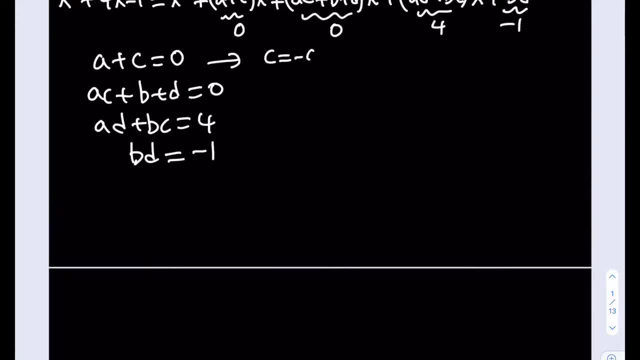 c here. How we can do that is well, we can just go ahead and replace the c with negative a. right from here, C is equal to negative a. so if you go ahead and plug in negative a, b plus t is going to equal a squared from here. If you replace c with negative a, you're going to get a d minus. 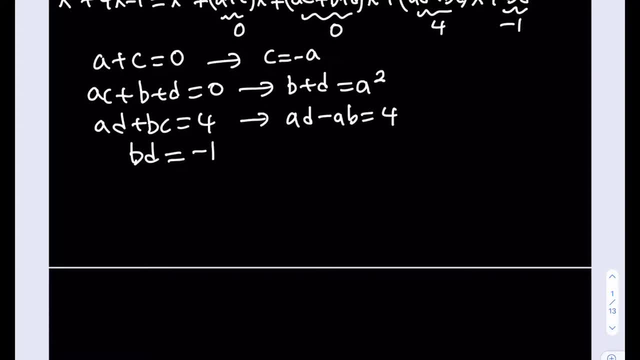 a, b being equal to four, and from here actually I can just go ahead and pull out the a That's going to give me a times. the quantity d minus b is equal to four, and from here I can actually isolate d minus b, because I have b minus b plus d, and if I can get the d minus b from here, 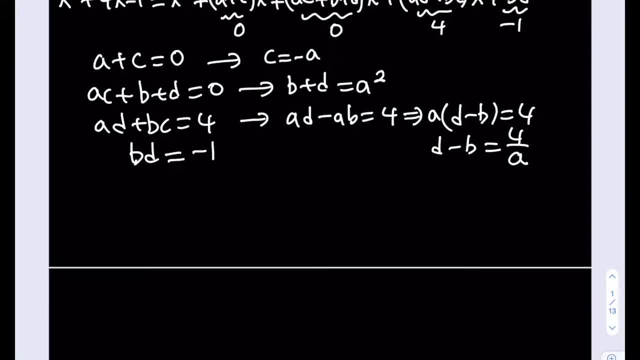 that's going to be helpful. So d minus b is going to equal four over a and, as you know, b- d is equal to negative one. So this is really cool because I got an equation basically on b and d like three different equations: one of them is numerical and the 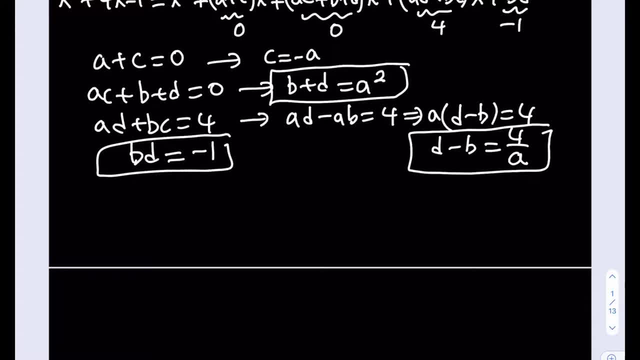 other one depends on a, So we should be able to work with this: three variables and three equations. Now, from here, we can actually go ahead and write d in terms of a because, and b in terms of a because, if you add these two equations up, okay, Let's go ahead and write it down here. 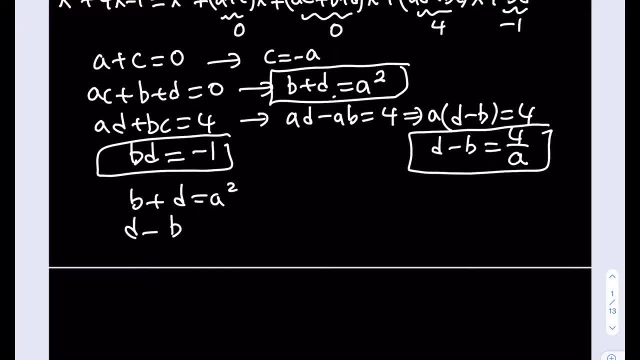 b plus d is a squared d minus b, riding down a according to my equation: promotion plus n, angle b plus d is a squared d minus b. b is 4 over a. We're just going to go ahead and add them up. The b is going to cancel out. We get. 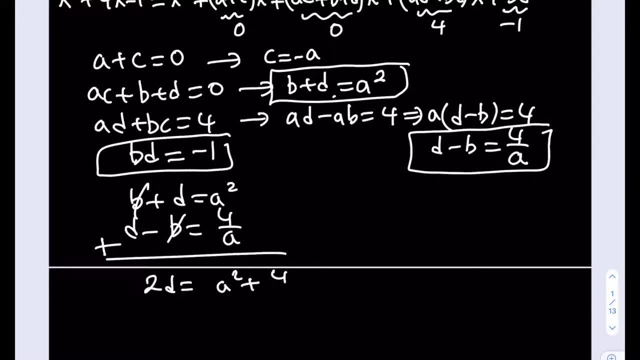 2d is equal to a squared plus 4 over a, and then from here we can actually go ahead and divide both sides by 2 and we'll get d in terms of a, which is going to be a squared over 2 plus 2 over. 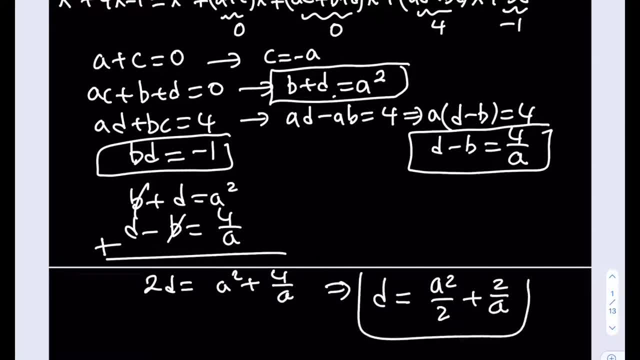 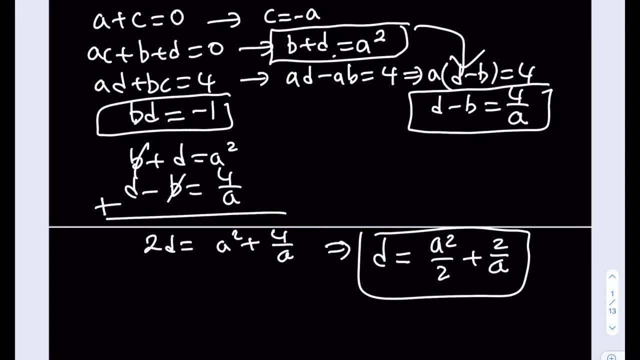 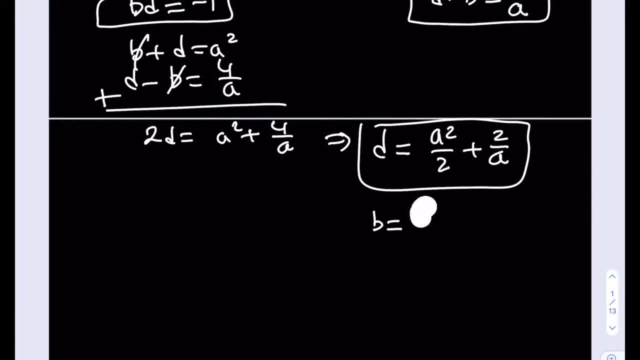 a. So this gives us the value of d in terms of a, which is nice. and then let's go ahead and find the b. and to find b, you can actually go ahead and subtract these equations side by side. That's going to be easier somewhat, and from here you're going to find that b is equal to a squared. oops. 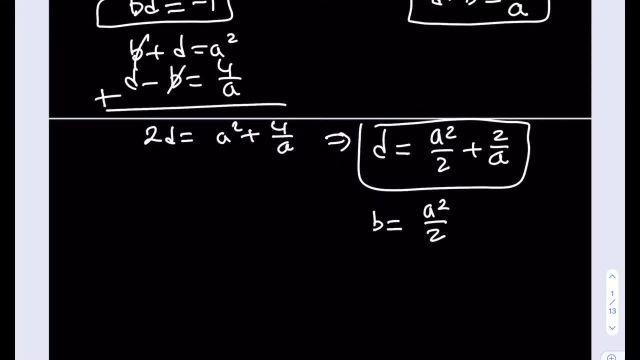 a squared over 2 minus 2 over a, So they're going to be like kind of conjugates. okay, All right, awesome. b and d are given like this, and we also know that b times d is equal to negative 1. So that's also cool, right? So what we can do is we can actually go ahead and multiply. 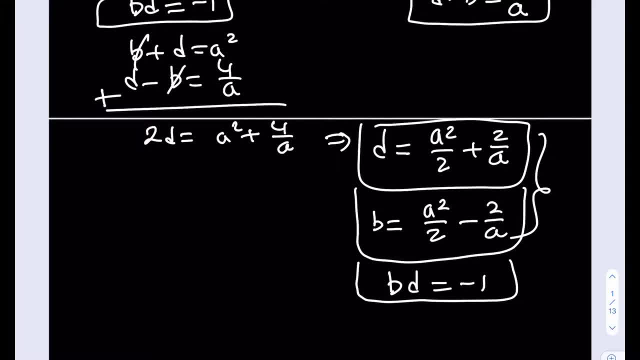 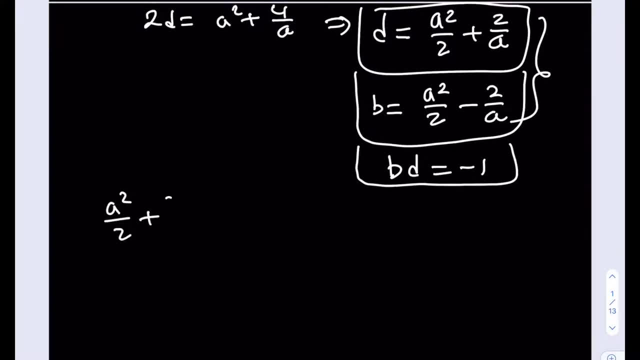 these two quantities in terms of a and then set it equal to negative 1 and then solve for a from there. Let's go ahead and do that a squared over 2 plus 2 over a, multiplied by a squared over 2 minus 2 over a, is equal to negative 1.. This is difference of two squares. so we're going to be. 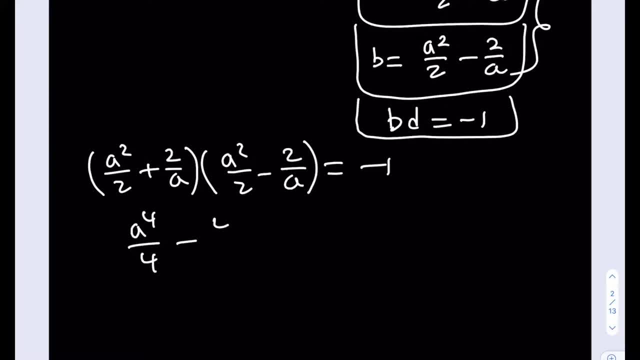 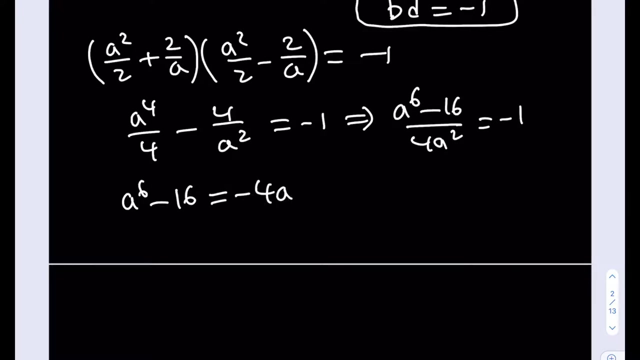 getting a to the fourth: power divided by 4 minus 4 over a squared is equal to negative 1. If you make a common denominator here, multiply by a squared and multiply by 4, you're going to get the following: and if you cross multiply, you're going to be getting a really nice equation. Well, not super nice, but we'll figure it. 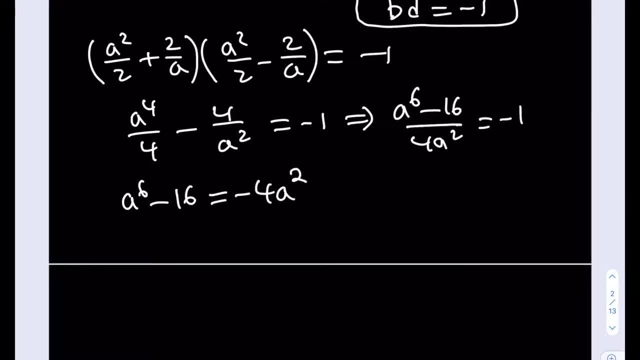 out right, We're going to find a way to solve it. Well, this kind of looks like a six degree equation, but we can actually simplify it because these are even powers. So we can go ahead and write it like this: first a to the sixth power plus 4 a squared. 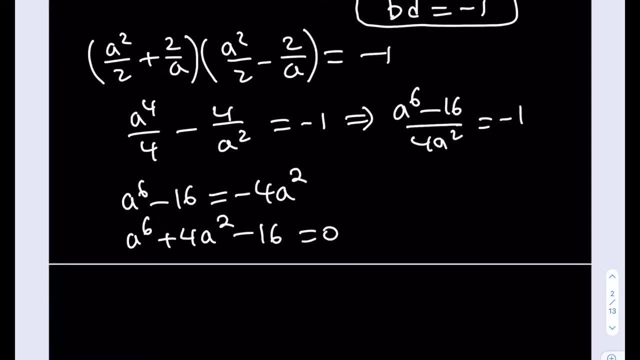 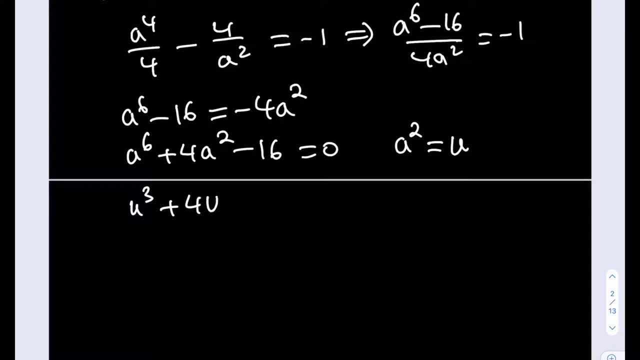 Minus 16 is equal to 0.. So let's go ahead and call a squared u, Then we're going to get u cubed plus 4. u minus 16 is equal to 0.. Now, using the rational root theorem, by checking divisors of 16, we actually find out that u equals 2 is a solution. 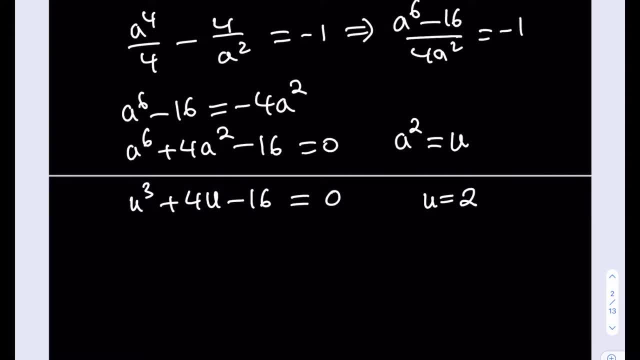 Okay, and if you divide this polynomial by u minus 2, you're going to find the other solutions. but the other roots are complex, so you don't really need to worry about them, because we're interested in real solutions here. So u equals 2, meaning that a squared is equal to 2, which means a is equal to. 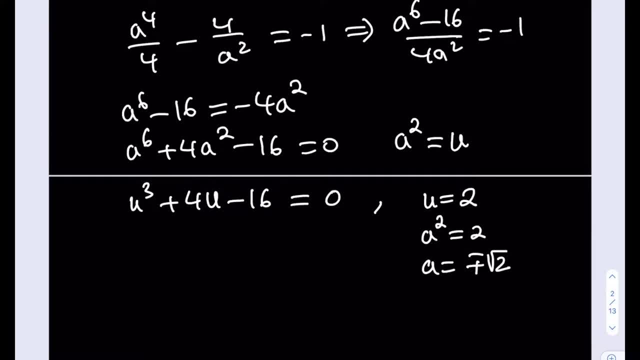 plus minus root 2.. Great, So we found the value of a, and a lot of things depend on a. First of all, we know that c is the opposite of a right. So we know that c is the opposite of a right. So we know that c is the opposite of a right. 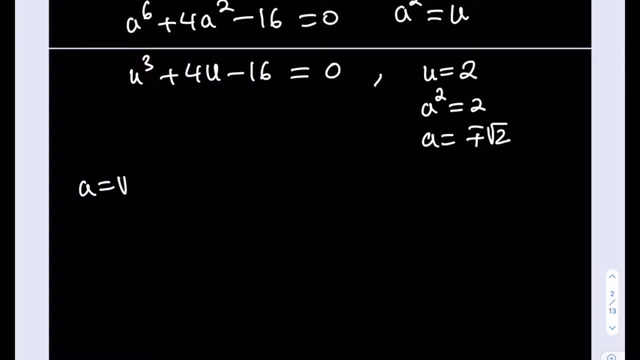 So, for example, if we take a is equal to root 2, which is one of the possibilities, Then from here we get that c is equal to negative root 2, because they're opposites, right. And then from here we get, d is equal to now. If you remember that we had b and d in terms of a. So 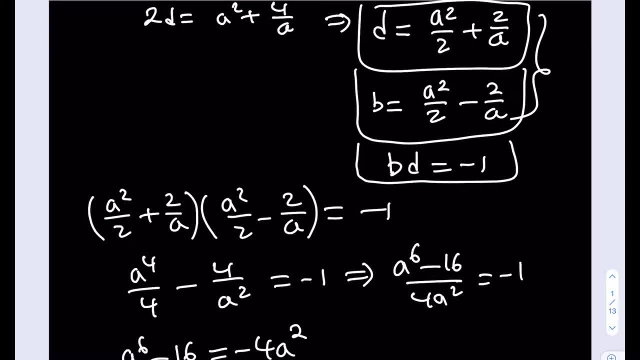 if a equals 2, for example, d is going to be 2 squared divided by 2, plus 2 over 2, right, And from here we're actually going to get the. I'm sorry if we take a equals root 2, root 2. 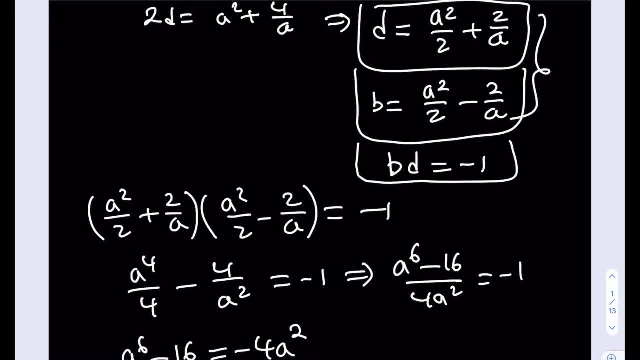 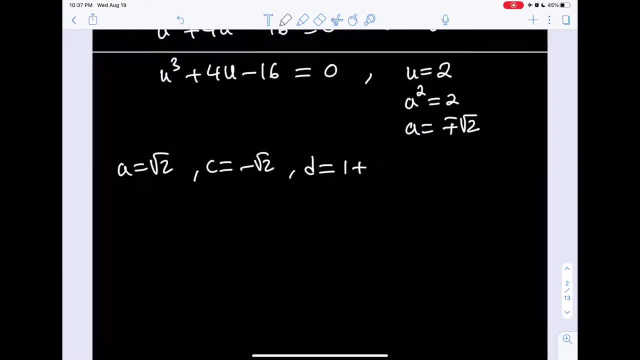 squared is: 2 divided by 2 equals 1.. 2 divided by root 2 is root 2.. So it's going to be root 2 plus 1. in other words, Okay, to keep a long story short, d is going to be 1 plus root 2 from here, right. 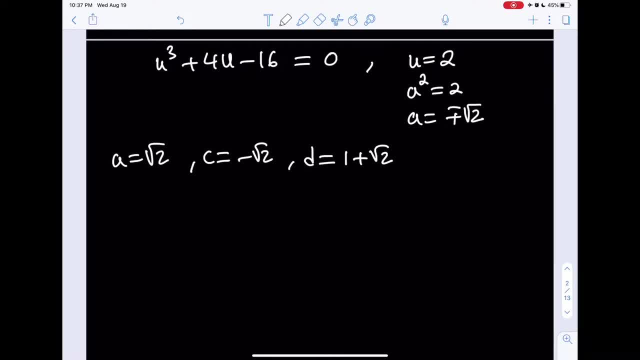 Okay, and then b is going to be 1 minus root 2.. We know that they are conjugates, so they're going to look like this: Okay, so we basically found the a, b, c, d values right by taking a equals root 2.. 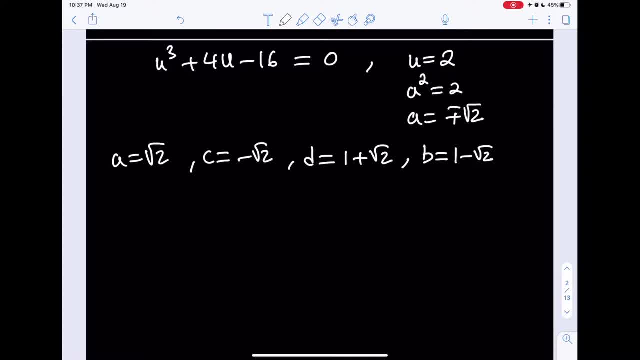 Obviously, by taking a equals negative root 2, you're going to be getting the other solutions which basically, they're just going to be switched around right. So our polynomial, eventually, is going to look like this: after factoring, It's going to look like this: We're going to get x. 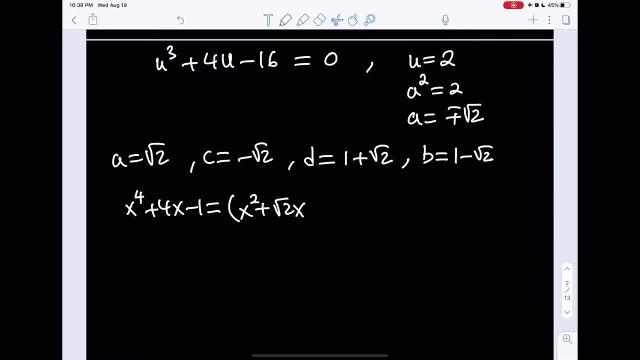 squared plus root 2, x plus 1 minus root 2, multiplied by x squared minus root 2, x plus 1 plus root 2.. And by setting each factor equal to 0, because they these are quadratics, we're going to be able to find: 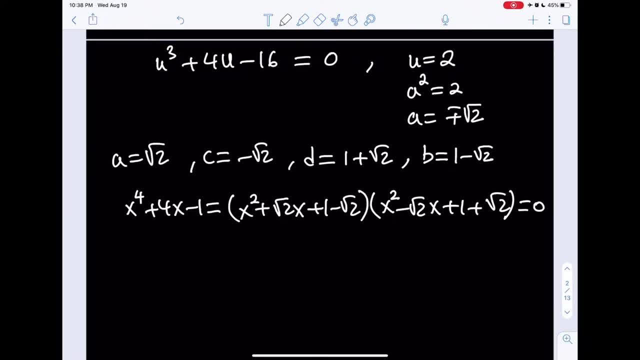 actually all the solutions. Okay, and how do you find the solutions from here? Basically, you can just go ahead and use the quadratic formula and you'll get the solutions. So let's go ahead and do that x equals. from here, we're going to be getting negative b plus minus the square root. 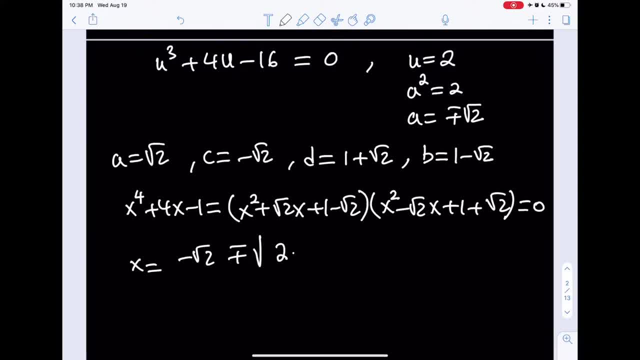 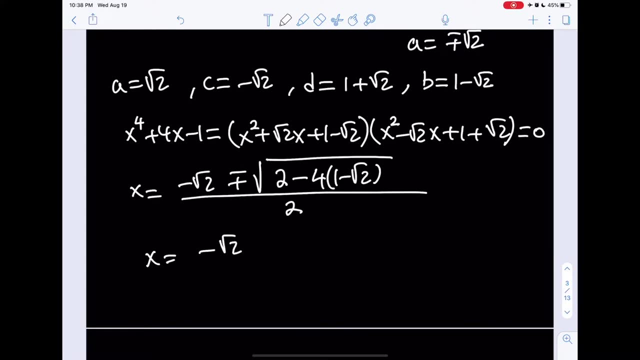 of b squared, which is going to be 2, in this case, Minus 4ac, That's going to be 4 times this quantity, Okay, divided by 2a, which is 2.. And if you simplify this a little bit, you're going to notice that it's going to be: x equals negative root, 2 plus minus. 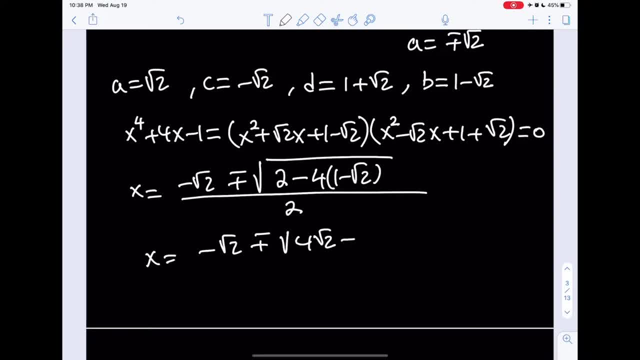 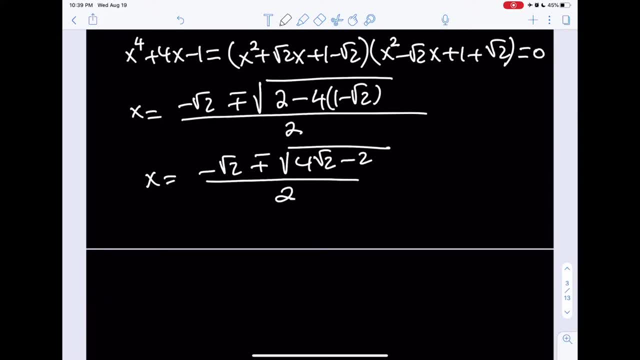 4 root 2, the square root of that, minus 2 divided by 2.. And the other one is basically going to give us, because this is a quartic, this is going to be, this is going to have four solutions here And the other solutions are going to be coming from the. 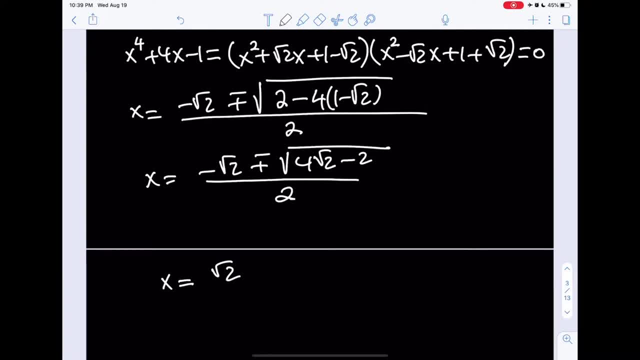 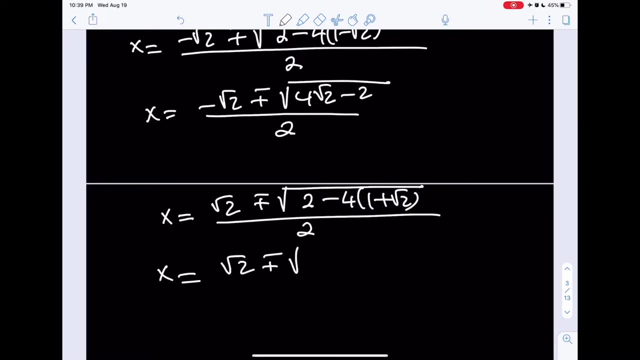 other equation which is negative: b plus minus the square root of b squared minus 4ac. Okay, and if you go ahead and simplify that, we're going to get something similar and we're going to obtain all the other solutions. Okay, all right, and when you distribute this, this is basically going to be: 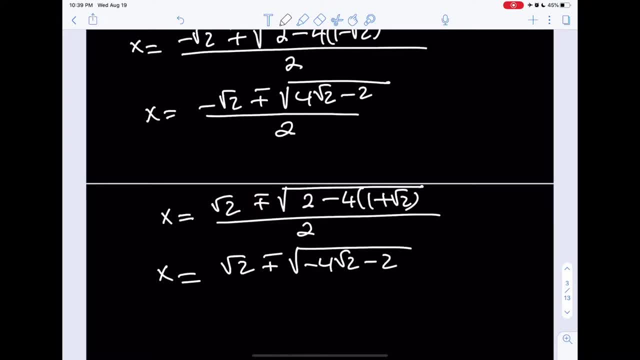 negative 4 root 2 minus 2 and divide by 2.. So obviously these roots are going to be complex because this is a negative quantity, square root of that is not going to be real, so on and so forth. So we're not really. I mean, we could just take them as complex solutions. 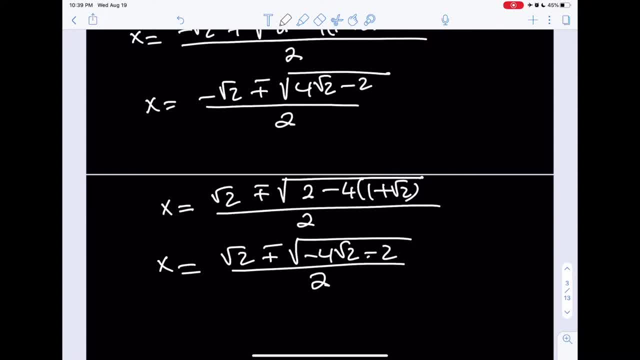 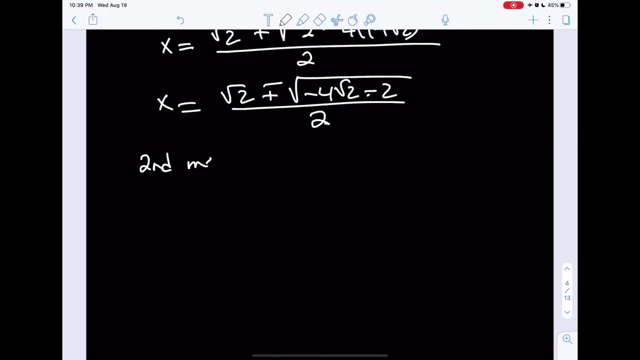 but that's pretty much it. Okay, that was our first method. Now let's go ahead and take a look at our second method, which is actually actually pretty interesting. I find it quite interesting. Obviously, the first one is like a brute force method, but second one is actually a really cool. 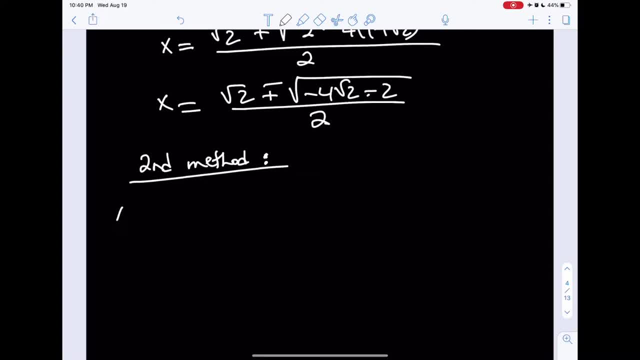 way to approach the problem. Okay, so our original problem is x to the fourth plus 4x, so I'm going to be adding and subtracting some terms to this to make it factorable. and how can I make most of these things factorable? You've probably seen similar problems like: okay, x to 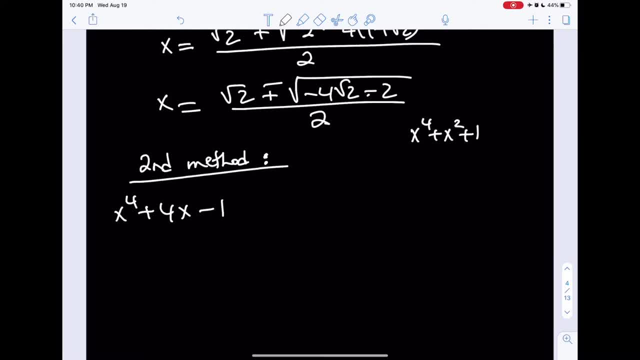 the fourth plus x, squared plus 1, is factorable because you can complete the square and turn that into a difference of two squares, or if you have something like x to the fourth plus 4 again, So with fourth powers, especially if there's a coefficient of 4 in there as well. 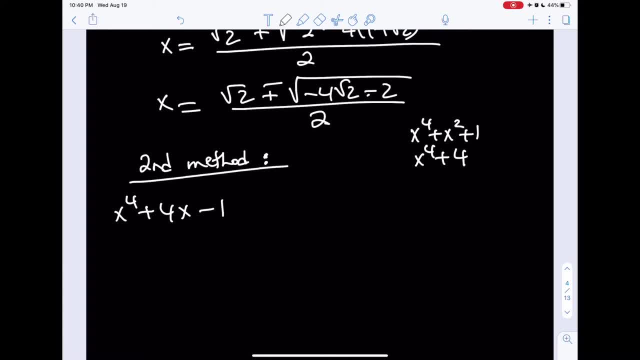 difference of two squares works really nicely. So this is what I'm going to do. I'm going to turn this into x to the fourth plus 2x squared plus 1, which is x squared plus 1, quantity squared right. but then I kind of need to arrange the other. 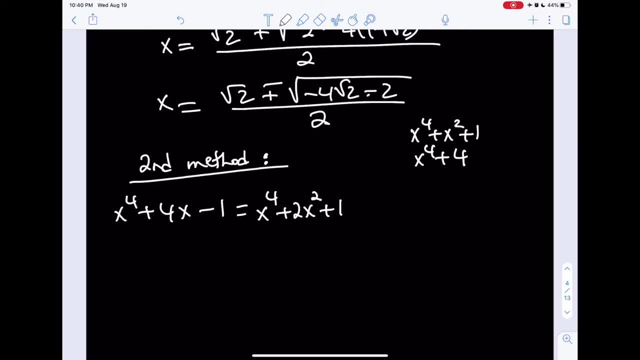 terms and the other terms are going to be like this: Okay, so I have a 4x, right? let's see what I added and what I need to subtract. So I added a 2x squared plus 1, so I need to subtract those. 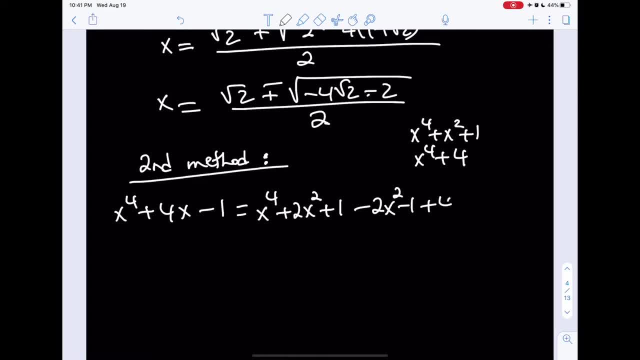 right and then write everything else. So let's see what this looks like. Then I'm going to be getting from here x squared plus 1 quantity squared, So hopefully I'm also going to be getting a perfect square from here. This is going to be: 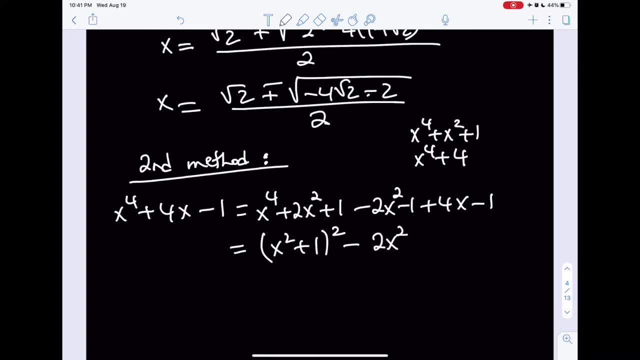 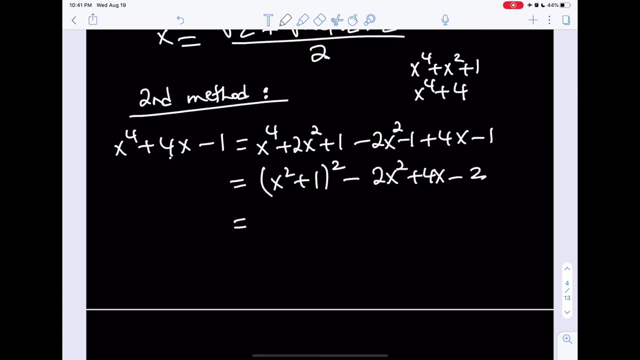 minus 2x, squared okay. plus 4x minus 2, right, okay. So what I did was I added 2x squared plus 1 and I subtracted it, and I then I just added these two terms, So everything looks good, right, Okay. now this expression, if you. 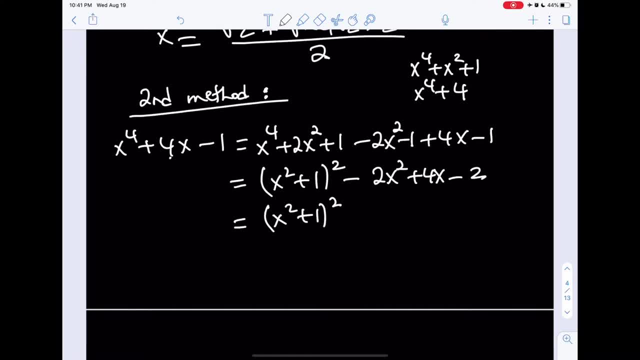 kind of factor it out. you're going to notice that this is actually factorable. We can take out a 2 there. The negative 2 gives us x squared minus 2x plus 1 and yay, this is factorable. nice, Okay so. 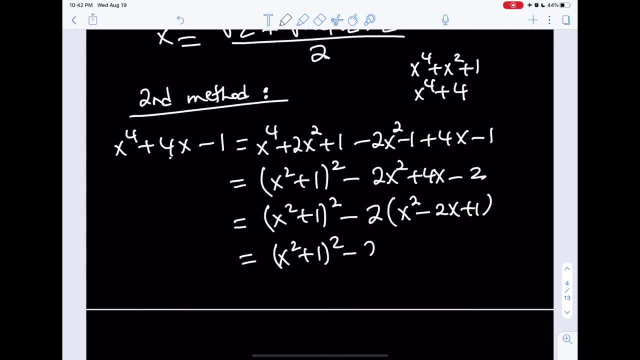 this is going to turn into x squared plus 1 squared minus 2 times the quantity x minus 1 squared. Okay, awesome, We were able to write it this way, but how is this factorable? from this point on, It's a difference of. 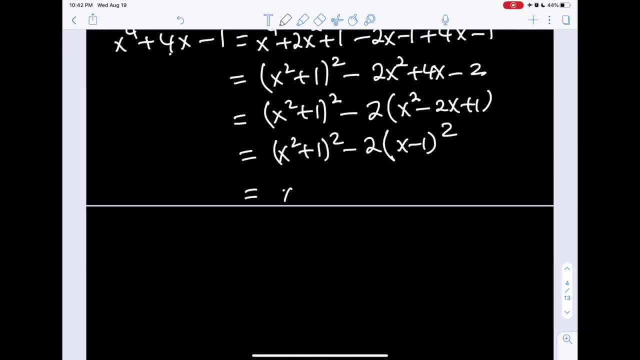 two squares, but two is not a perfect square, but that could be taken care of. So we're going to be writing this expression as this: Root 2 multiplied by x minus 1, and that quantity is squared. There you go. Now we got a difference of two squares. we can just go ahead and factor it: a plus b.